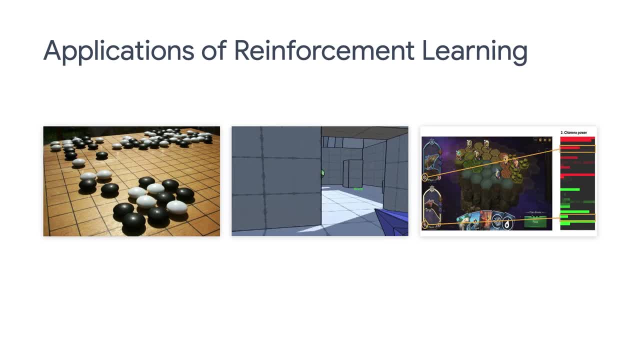 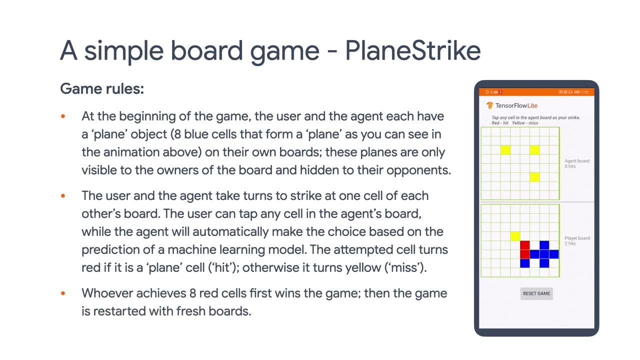 Gaming is a hot testbed for reinforcement learning, for sure. So how do we leverage TF agents to build a game then We are going to show you today. The end result will be a simple board game we are showing here. The game is called Plane Strike. It's very similar to the Battleship game. 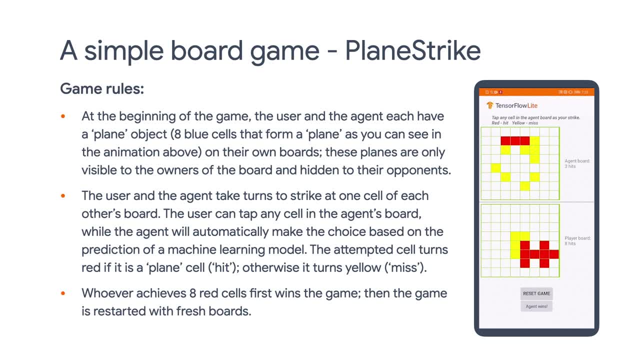 if you have played that one before. The rules are very simple so I won't read them out loud here, But at a high level. you play against an agent trained by reinforcement learning and your task is to guess out all the agent's hidden plane cells in blue before the agent. 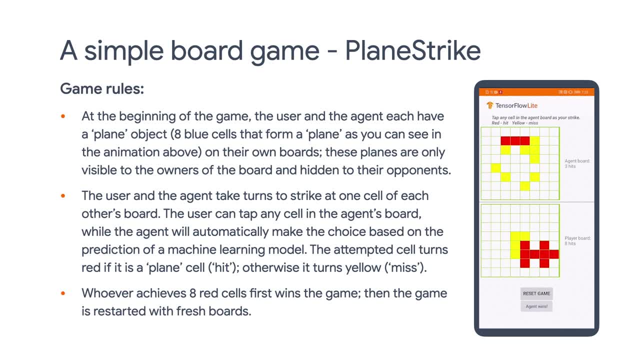 does to your plane cells. In order to make the game interesting and fun, we need to train a strong agent that can finish the game in as few steps as possible. To build such an agent, we are going to use a different kind of reinforcement learning algorithm. 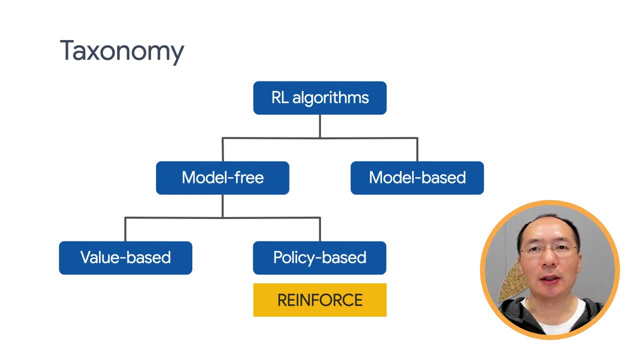 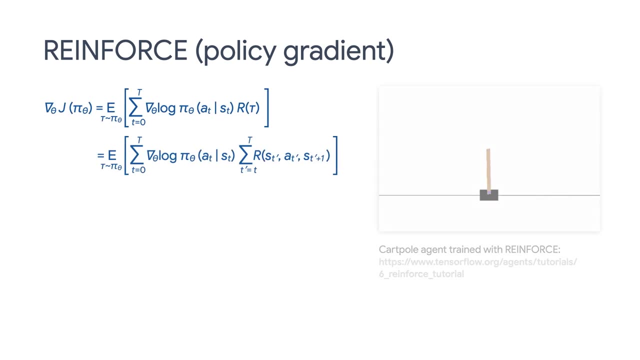 which is a policy-based algorithm. We call that. unlike the value-based algorithm DQN, which learns to predict the action state value, we are going to train a newer network to directly output the optimal policy. We won't go into the math here. 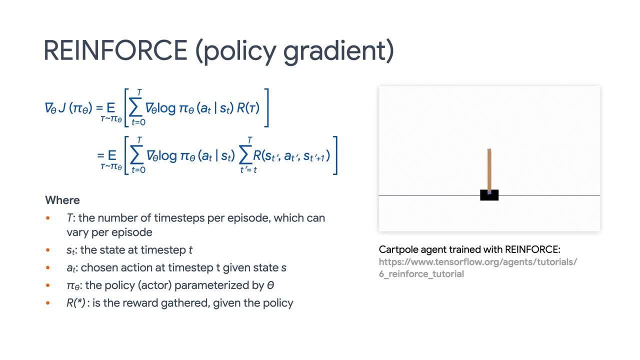 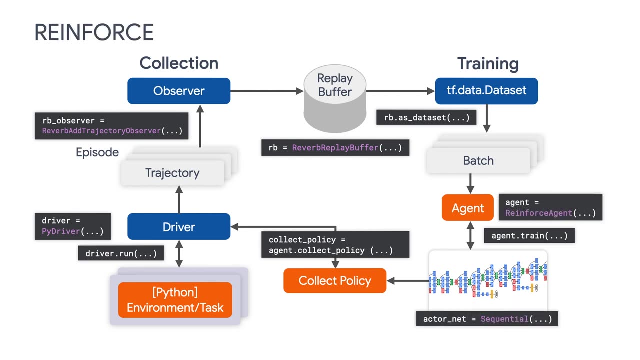 but the basic idea for reinforcement learning is to adjust the policy network parameters based on the reward signals collected during the gameplay so that the policy network can maximize the return in future plays. Overall, we are following the same workflow as in our DQN episode, But before we dive into training the game agent, we need to first create a training. 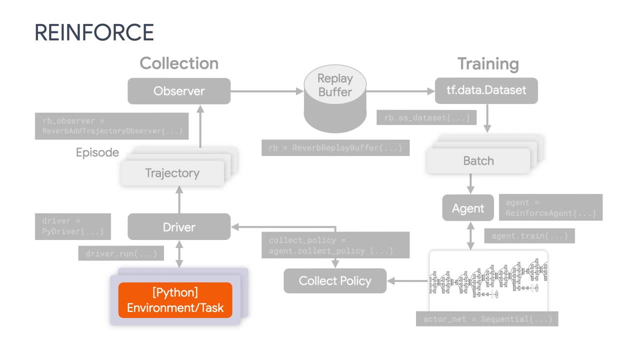 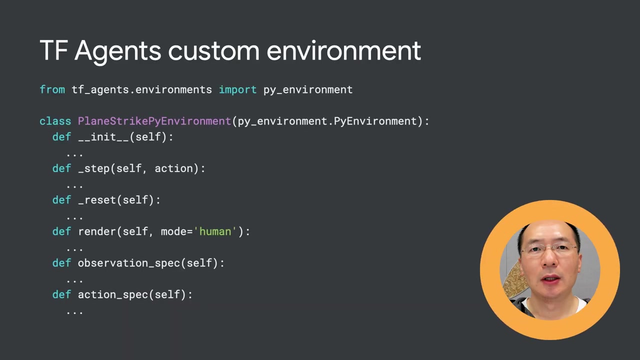 environment from scratch, since there's no existing environment for our own purpose. Although TF agents can directly import custom GM environments, we are going to create a TF agents environment this time, just to show you how to do this. The TF agents custom environment is actually pretty similar to OpenAI GIMP custom environment. 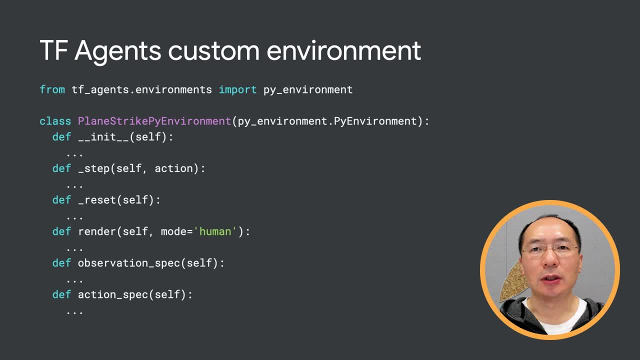 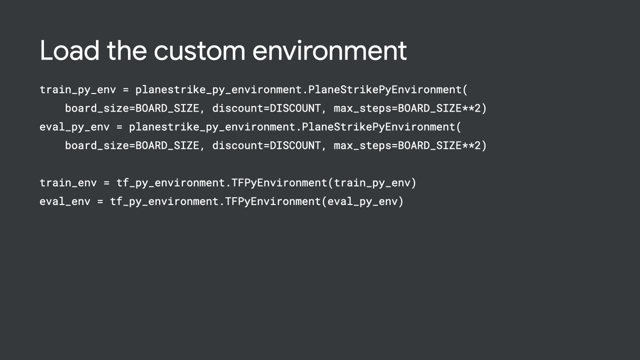 but we need to define 6 functions: Init, step, reset, render, observation spec and action spec functions. We won't go into the detailed code here, but feel free to check them out in the link here. After the environment is defined, we can easily import it, Unlike for the 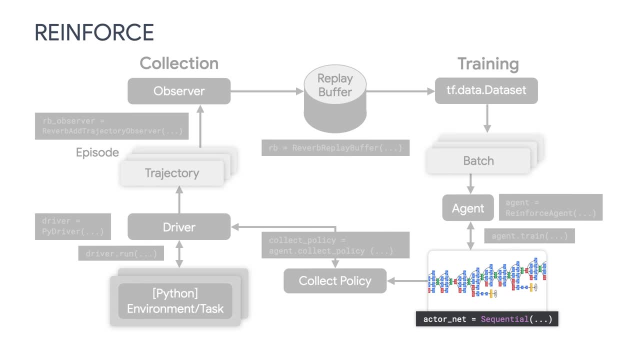 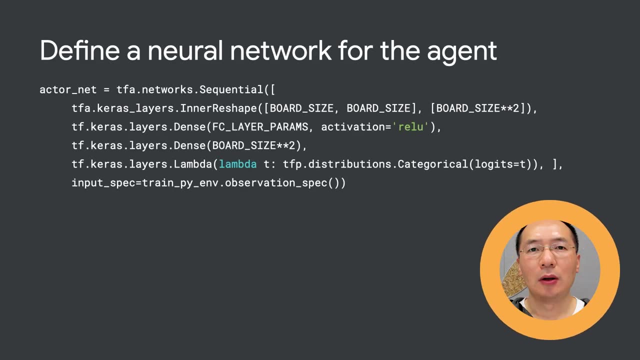 DQN agent we defined earlier. we can easily import it. This is the first step of the process. define a Q-network to predict the Q-value. here we define an actor network to represent the policy. We are using the familiar Keras sequential model. and the only thing I want to point: 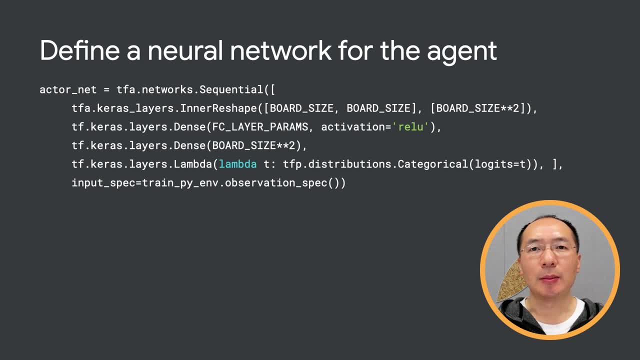 out here is that the last layer, a lambda layer that outputs a categorical distribution. This is similar to our DQM agent for CardPo. It's for discrete actions that can only be discrete numbers. We'll be discussing discrete versus continuous control in the next episode. 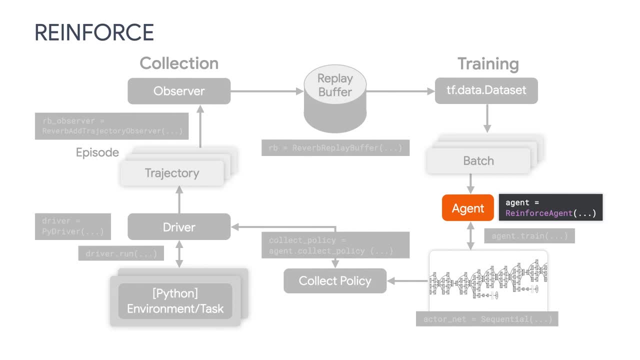 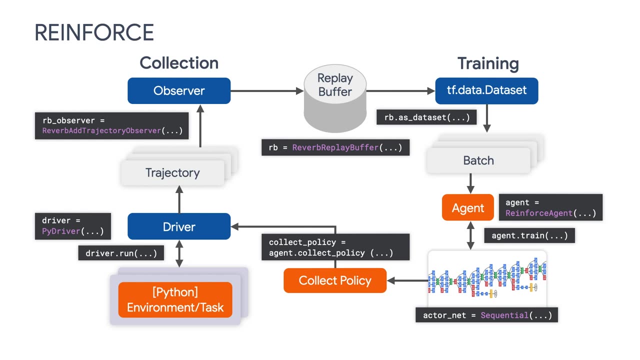 Next we are going to define our agents. Naturally, we're using Reinforce agent here. The other pieces are pretty much the same as in our previous DQM episode. There are a couple of places you need to change for the replay buffer, otherwise it's almost. 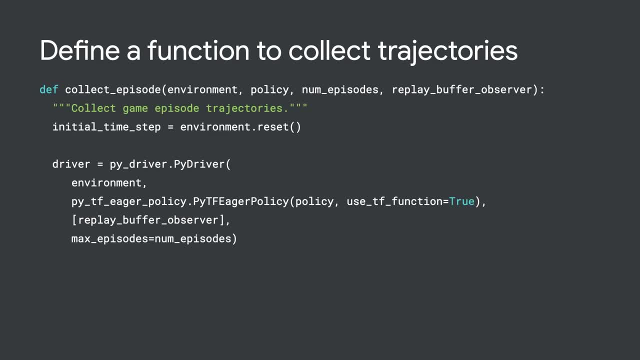 the same As Reinforce learns from the whole DQM. We define a function to collect an episode using the given data collection policy and save the data, which includes observation, action, reward and etc- as trajectories in the replay buffer. Finally, we run the training loop. 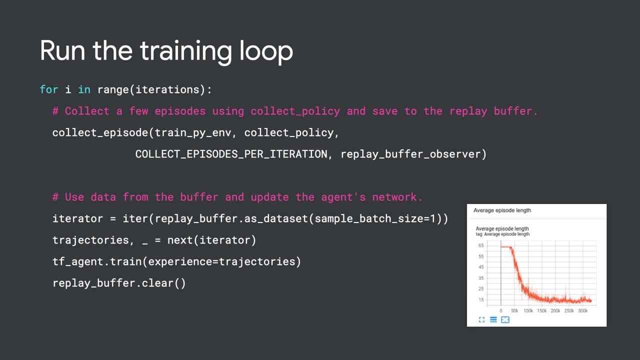 You can see in TensorBoard that the average episode length gradually decreases, which means our agent is becoming smarter. since we want it to finish the game as soon as possible so that it doesn't have to wait, It can beat the human player. 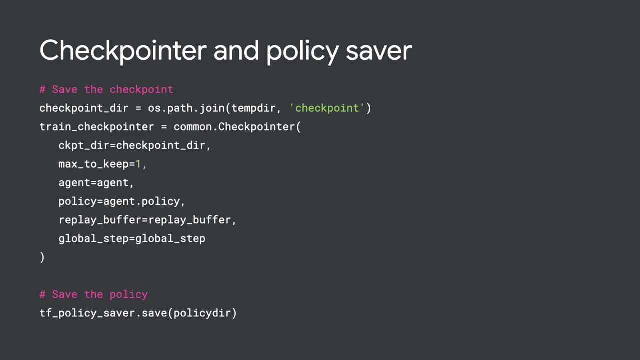 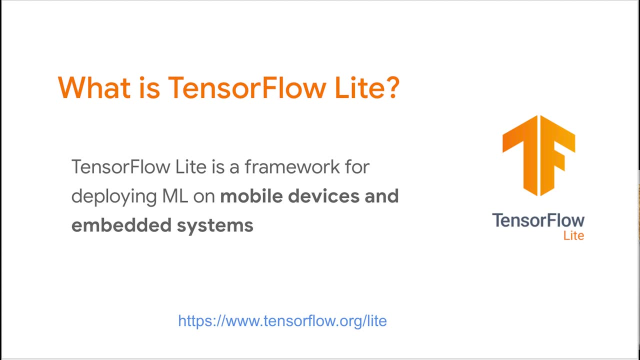 After training, we can export the policy as saved model for deployment using the policy saver, But we're building a mobile app. we cannot directly use saved model. This is where TensorBoard Lite comes in. TF Lite is a framework to run machine learning models on mobile and IoT devices. 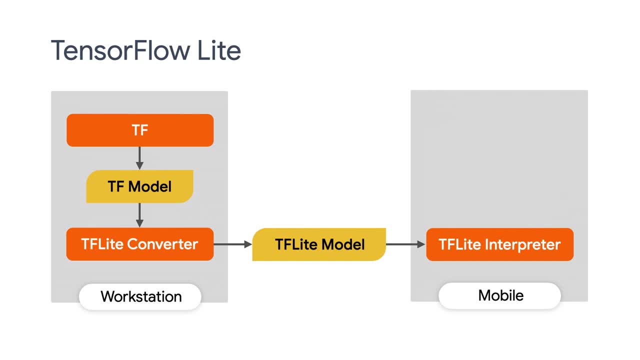 We won't go into details about TF Lite here, but the standard TF Lite flow is: first we use the TF Lite converter. We use the converter to convert the saved model to a TF Lite model and then we deploy the model into an Android or iOS app.